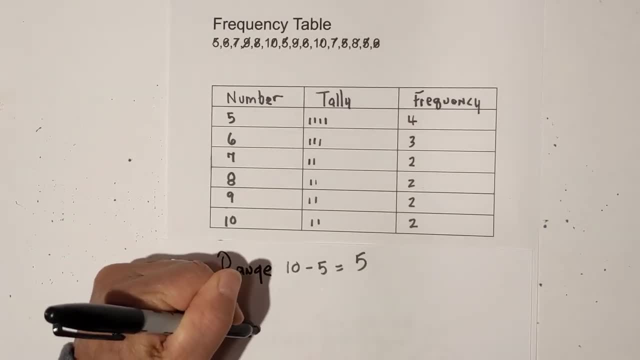 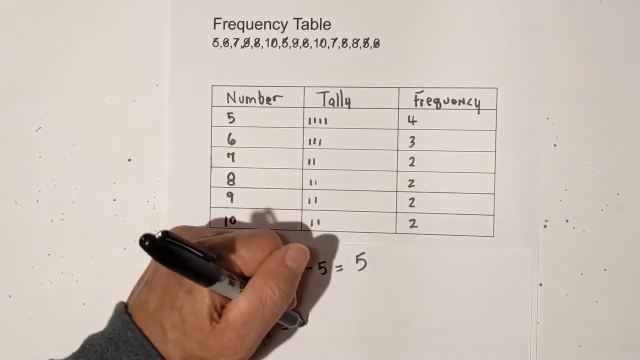 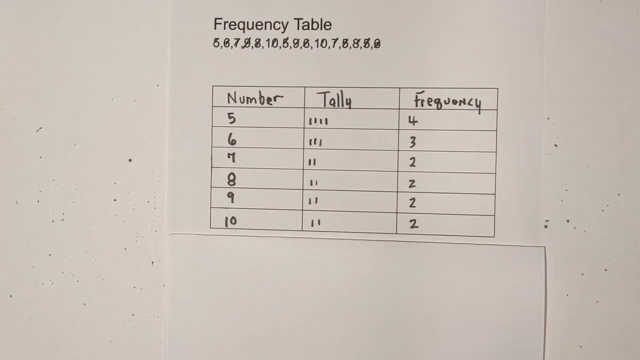 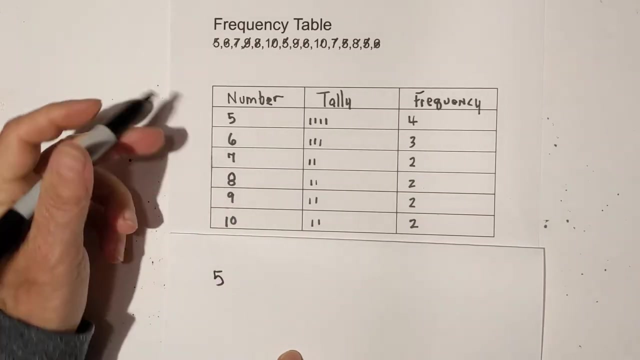 Next, the mode is just the number that appears most often in the data set, And so you just look at the frequency and 5 appears most often. 4 is the greatest. Now let's move on to the median. Now for the median. I think the easiest way of using a frequency table is just to rewrite your numbers from smallest to larger, and how many each appear. 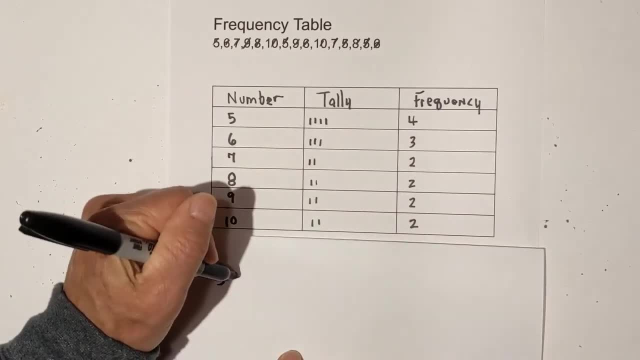 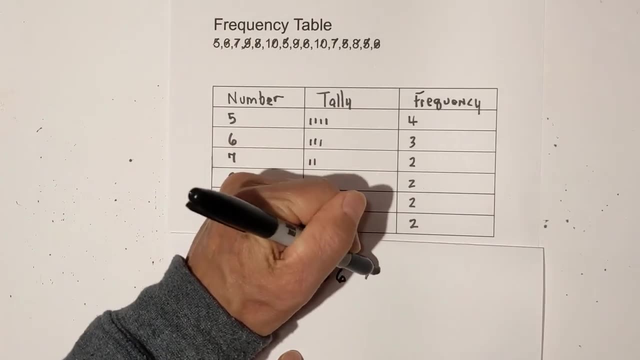 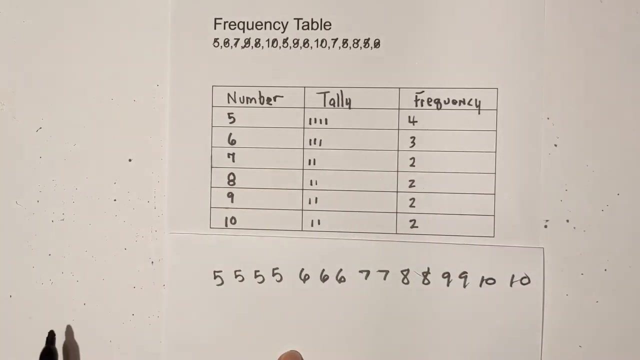 And so the frequency table gives you that data. So 5 appears 4. 4 times, Then 6 appears 3 times, And then the 7 appears 2 times, The 8 appears 2 times, Same with the 9 and same with the 10.. 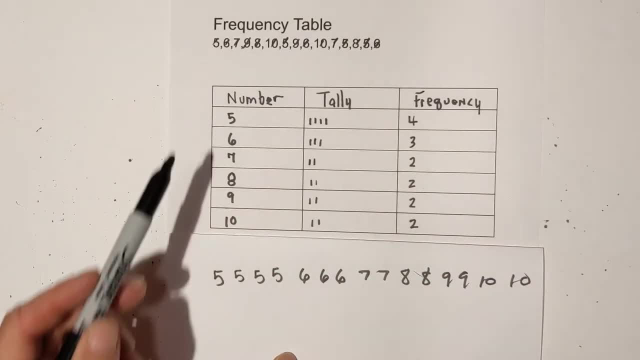 Okay, so you may want to double check. I know that I have 15 numbers, so I may want to count, just so I don't make a mistake: 1, 2, 3,, 4,, 5,, 6,, 7,, 8,, 9,, 10,, 11,, 12,, 13,, 14.. I do have 15 numbers. 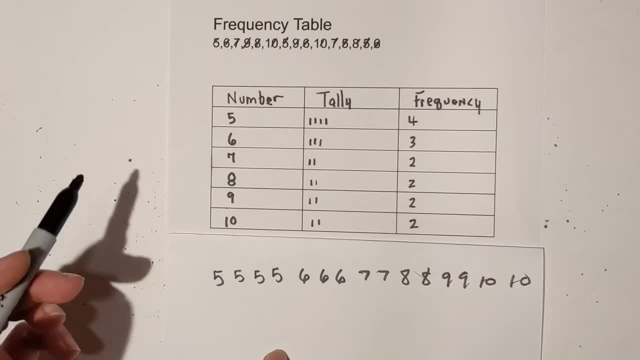 Now I just eliminate them because you, You know the median. Let me go ahead and write what we're looking for. The median is the number right in the middle. Okay, so I'm going to start eliminating. I'm going to eliminate one from this side, one from this side. See what I'm doing. 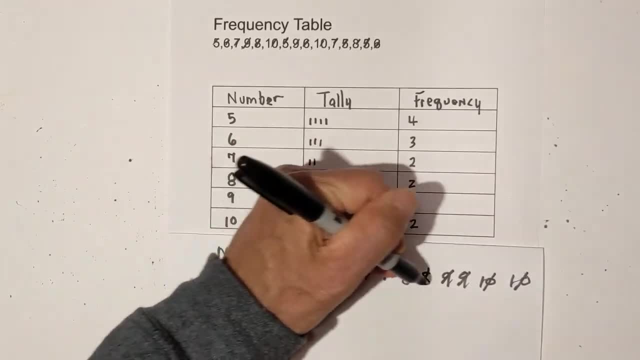 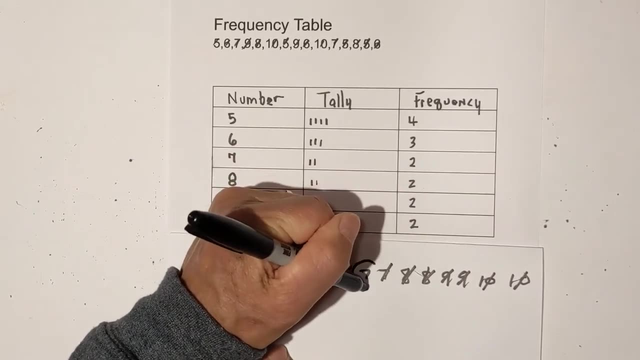 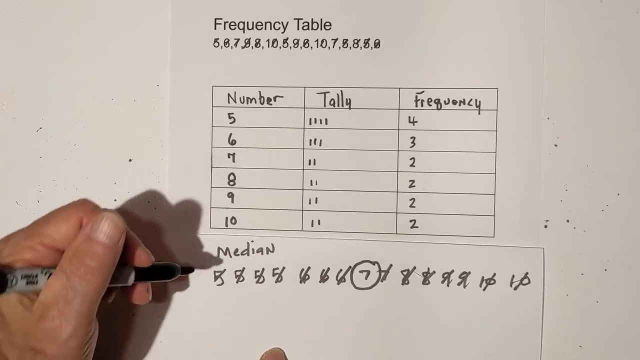 Okay, slowly go through each of these until I get the number in the middle And it is 7.. Now what if you have an even number and you get to the middle And there are two? Say, for instance, if I added a number 5 here, I would get to 6 and 7.. 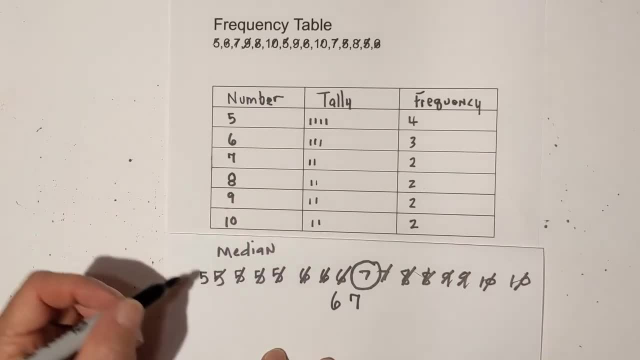 So what you do is you take the average of those two if you have an even number, But in this I have an odd, so it works out to where 7 is the median. Okay, now let's move on to the very last one. 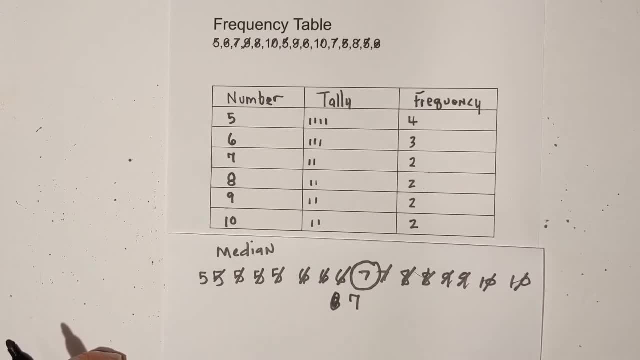 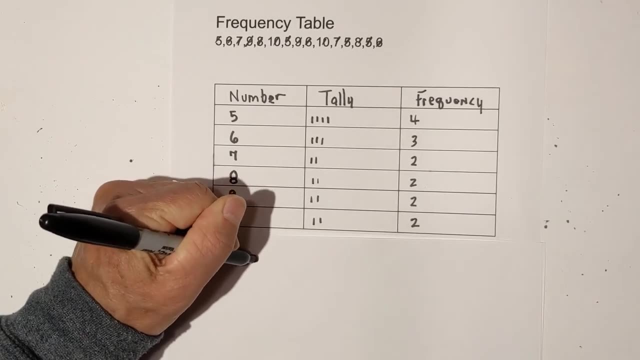 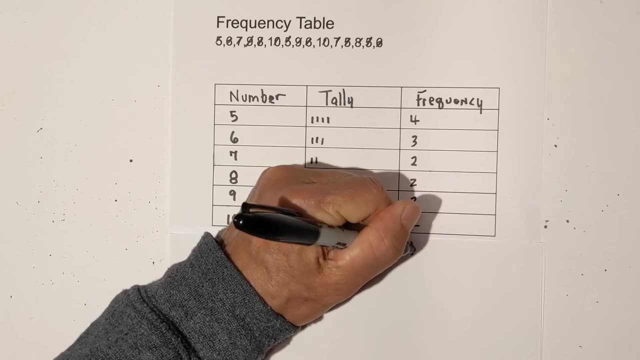 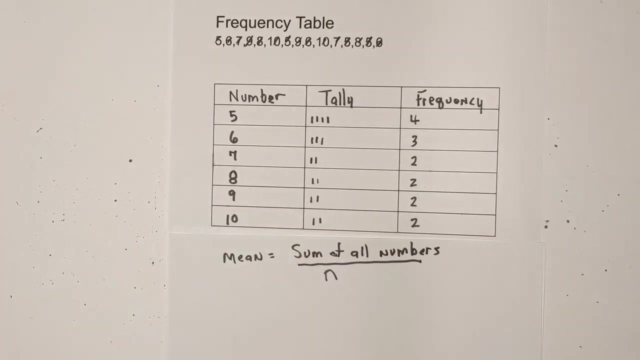 And that is going to be the mean, And we'll have to do a little bit of work for that. Now for your mean. the mean is equal to the sum of all numbers divided by n, which is the total of how many numbers you have in the data set.